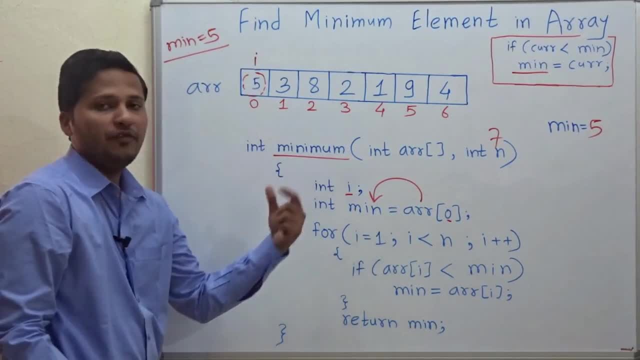 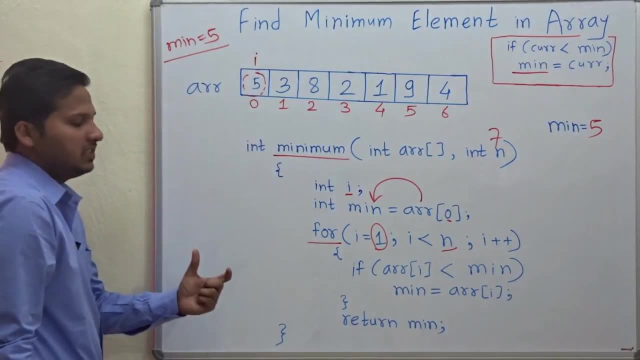 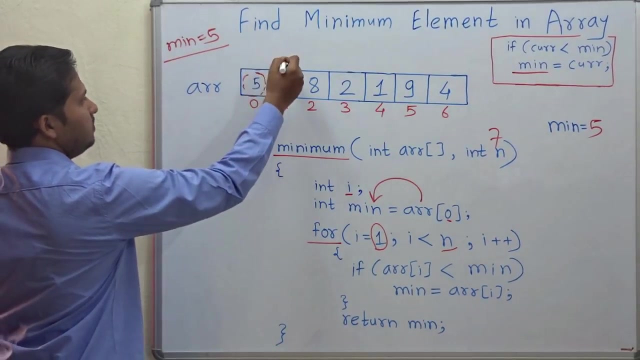 that allows the minimum element to be declared. So the minimum element is declared and the element is assigned to the minimum variable. Now let's start the for loop from the first index to the last index. that is n. Now see for i. equal to one means i will be one now. So if array of i is 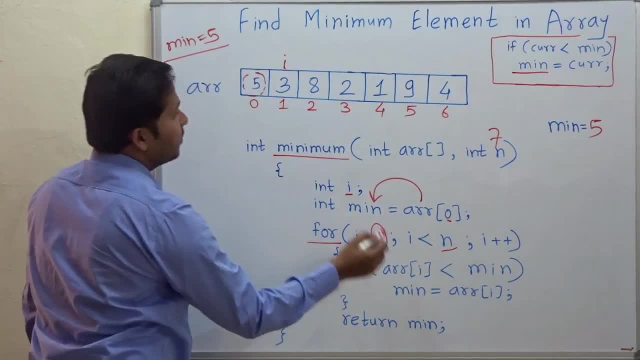 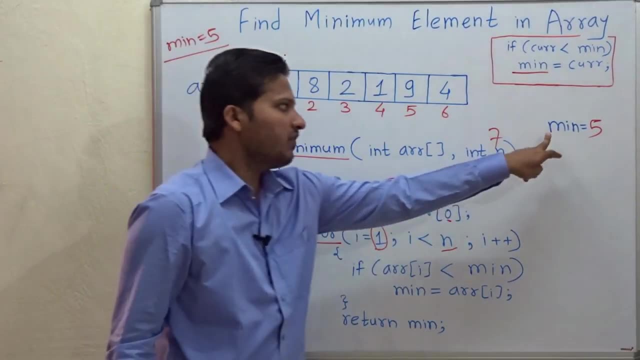 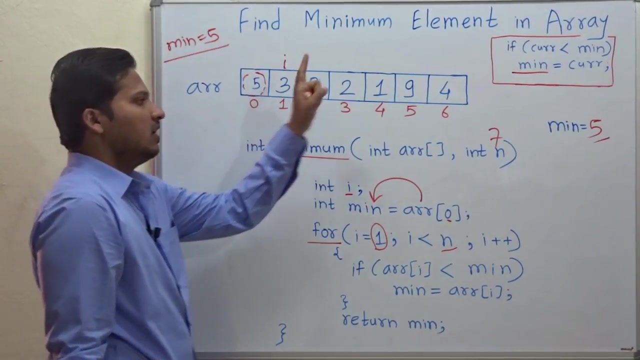 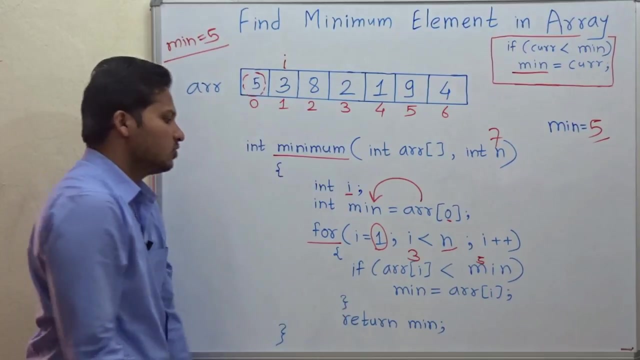 less than minimum means you have to check whether the current element is less than the minimum variable. Okay, this variable minimum is holding the value five now. So you have to check whether the current element three is less than five. See here, three is less than five. Yes, it is. So this if condition. 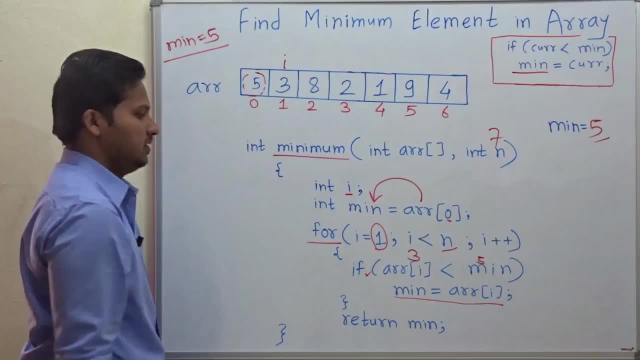 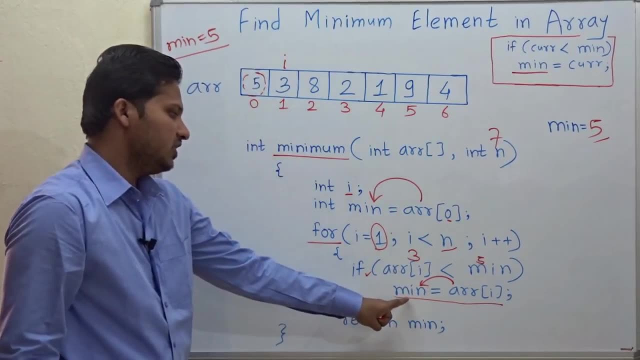 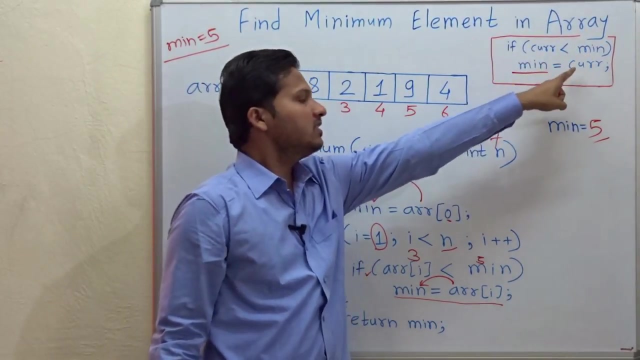 is true, And we go inside this if condition: Okay, And that current element becomes the new minimum inside the if condition. So see here, this is the rule: If current is less than minimum, then that current element becomes the minimum. Okay, means that value. 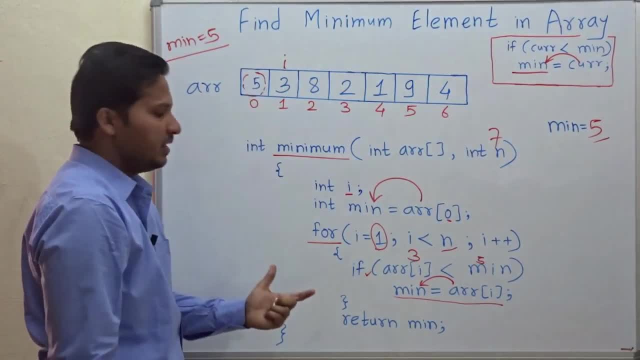 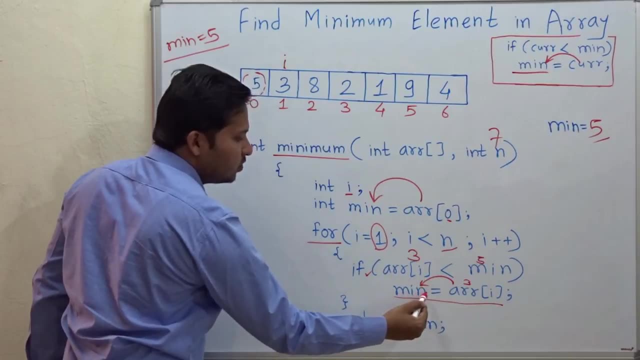 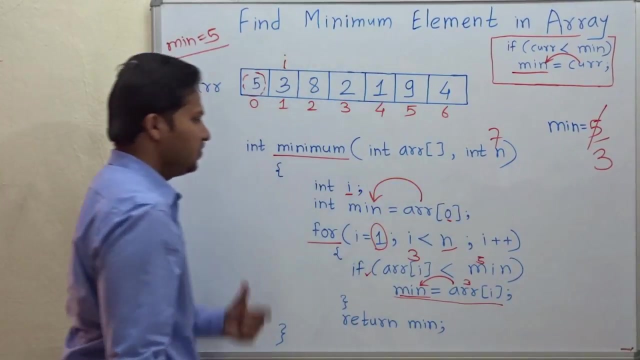 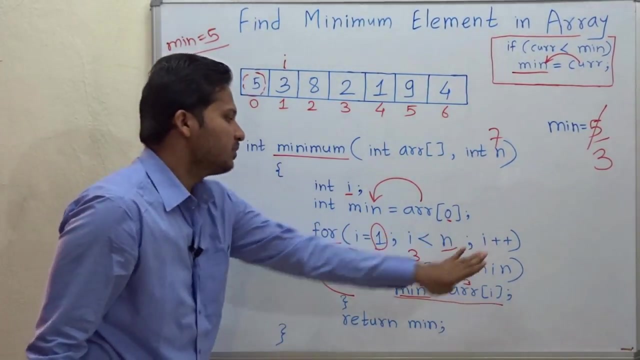 of the current element is assigned to the minimum variable. So see, because three is less than five, now three will be assigned to the minimum variable. Okay, so this variable is updated And now minimum is three. Right, And we go to the next iteration of for loop. Now i plus plus means I will become two now. So see whether eight here. 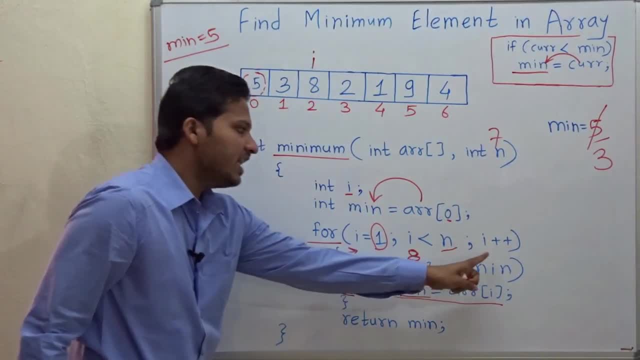 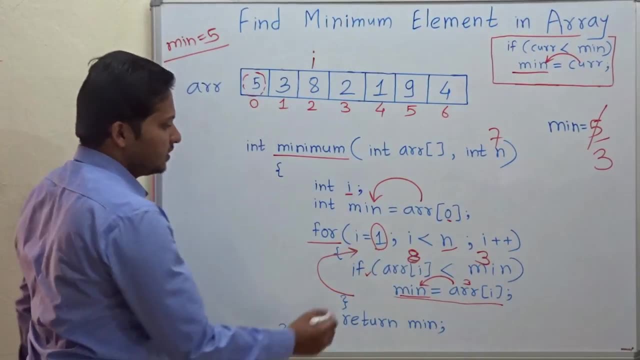 if array of i, that is, eight, is less than minimum. now minimum is three. Okay, so whether eight is less than three, No, it is not. So we don't go inside this if condition. we just directly go to the next iteration. 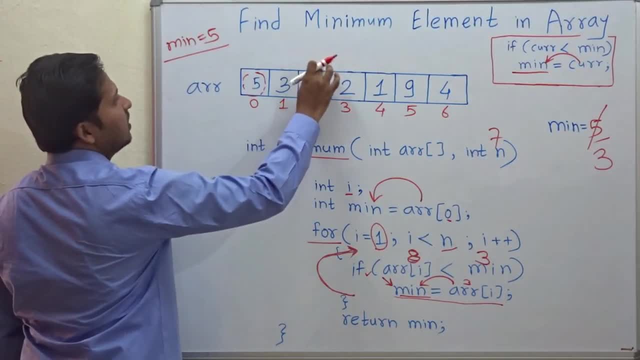 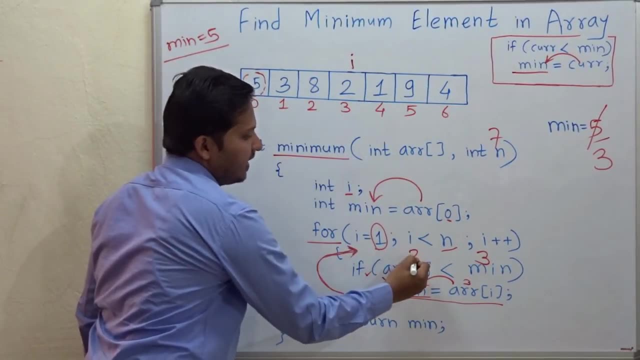 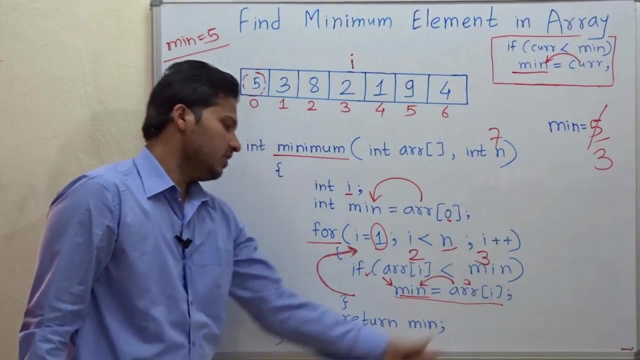 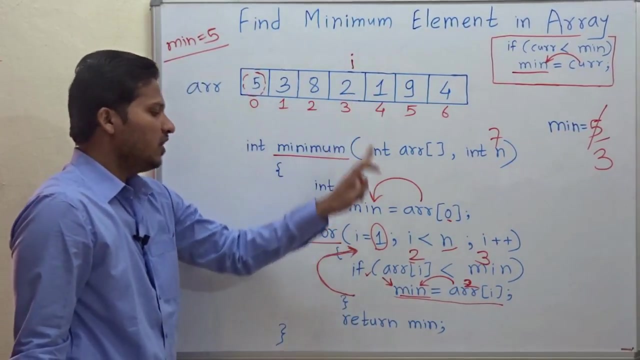 so I plus plus means we go to the next element. now check 2. so whether 2- that is array of I- is less than 3, that is the minimum. yes, 2 is less than 3, so 2 will be assigned to the minimum variable. now means the current element, 2 will become.